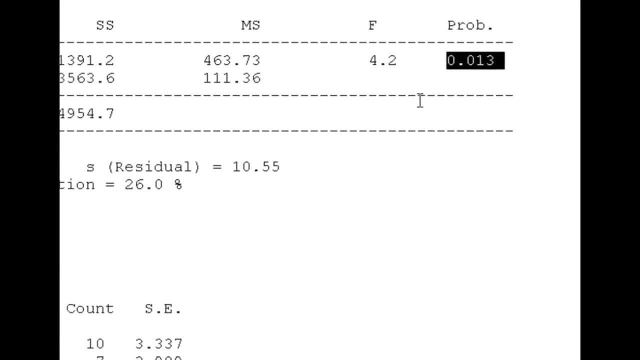 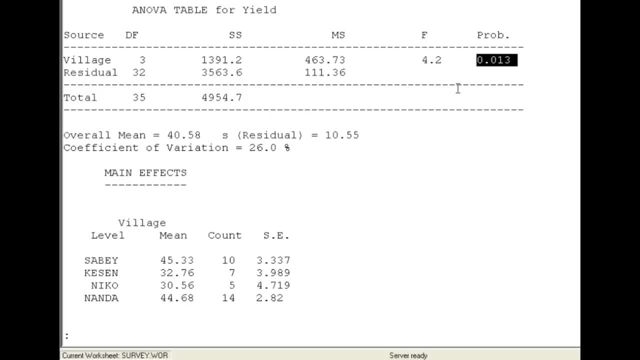 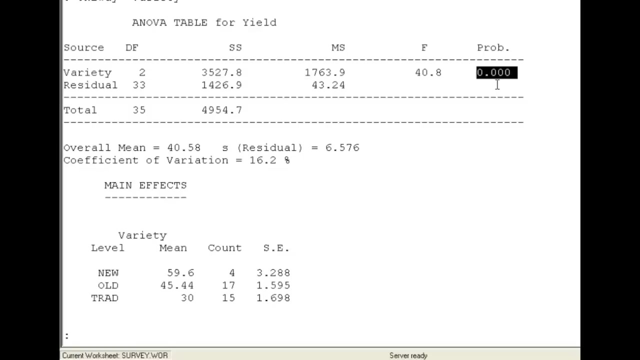 Now, this result isn't as clear as others we have seen, but does show some evidence to reject the null hypothesis in favour of the alternative. Let's try another example, this time with the varieties. The p-value this time is 0, or more precisely it's less than 0.001, ie less than 0.1%. 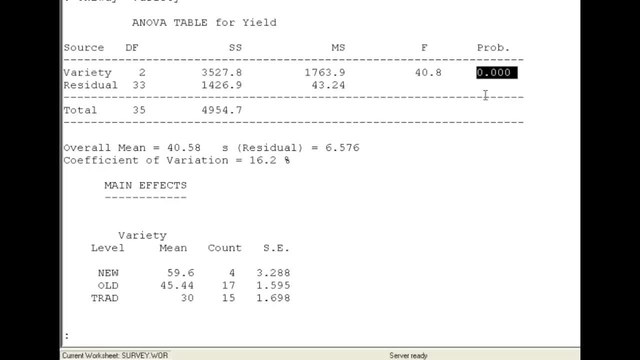 The result here is quite clear: The null hypothesis is rejected and we accept the alternative hypothesis that the true means for the varieties are different. The alternative hypothesis is very general and this significance test is a sort of passport to interpret the differences between the means. 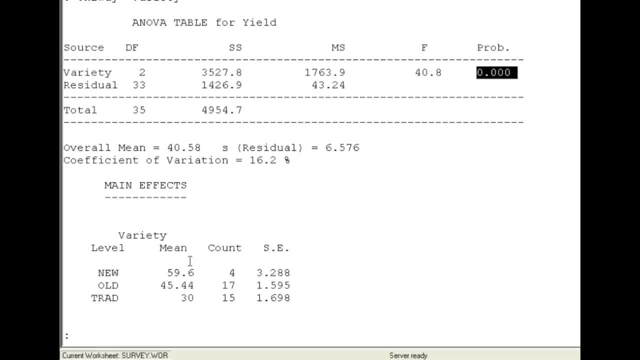 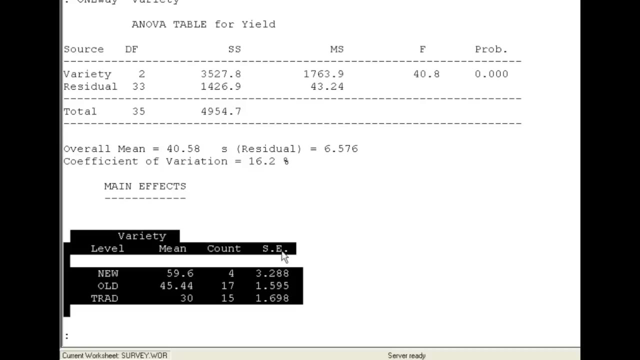 which are shown knowing that the differences are real. At the end of the results there's the table of means giving the mean value for each variety, the number of cases for each variety and the standard errors of the means. Just below the ANOVA table we have the overall mean. 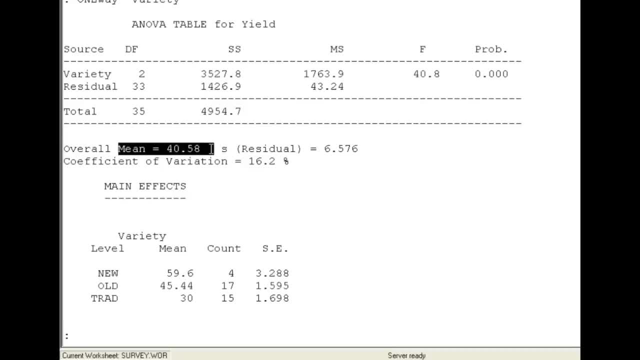 which in this case is 40.58.. Now the first column of the ANOVA table itself shows the degrees of freedom. The total degrees of freedom is 35,, as we have 36 records, and the total degrees of freedom is the number of records minus 1.. 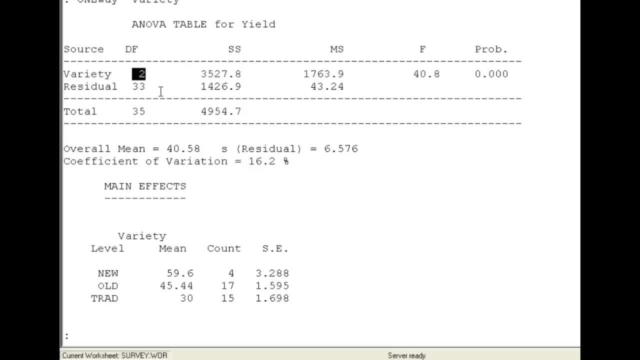 The variety has 2 degrees of freedom, as we have 3 varieties, leaving a residual or a leftover bit of 33.. The next column shows the sums of squares. The total sums of squares is 4954.7 and this is calculated by summing over all records. 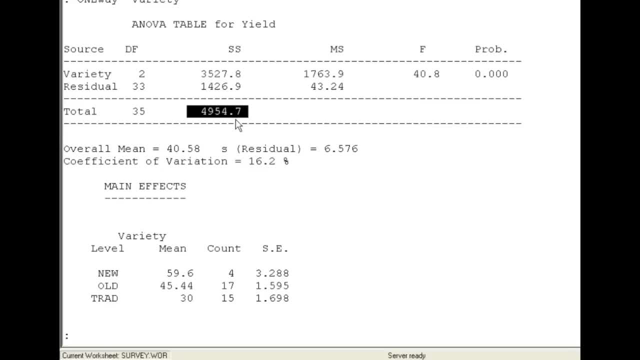 the square of the difference between the yield and the overall mean. The residual sum of squares is calculated in a similar way to the total, but this time we square the difference between each yield value and the corresponding mean for that variety, And this comes to 1426.9,. 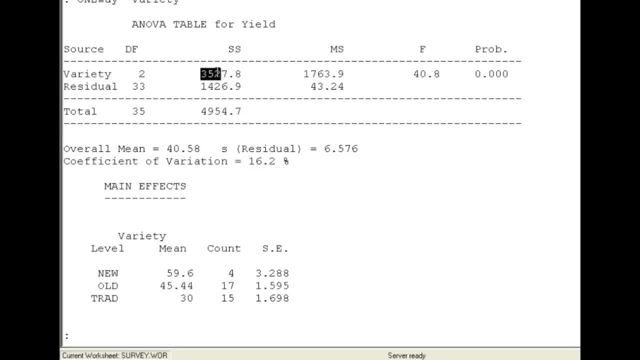 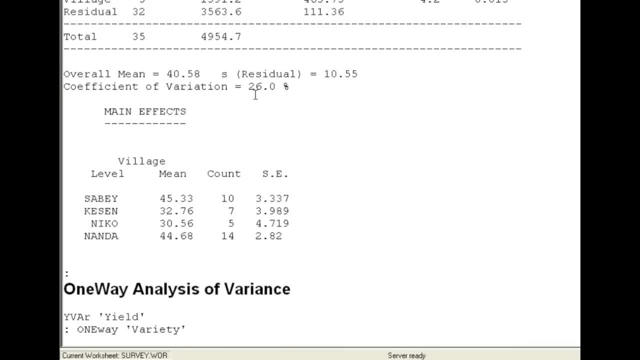 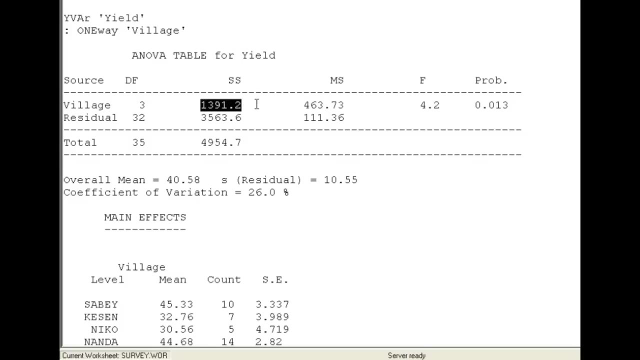 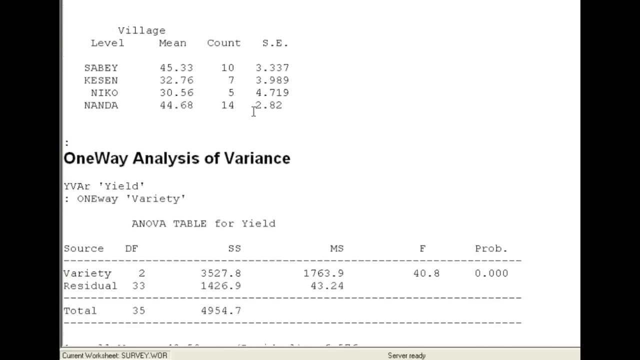 leaving 3527.8. that is explained by the variety factor. We can compare this to the results for the village and we find there's much less of the sums of squares is explained by the village factor: only 1391, as opposed to 3527.. 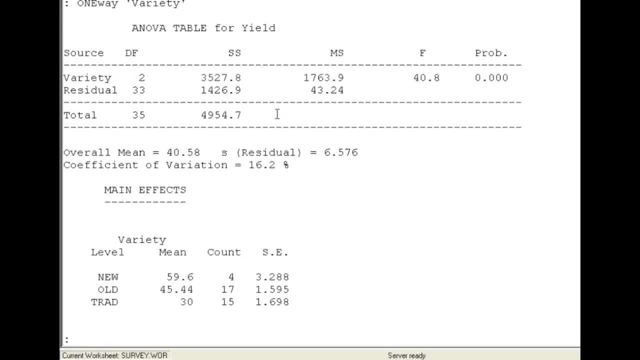 So it seems that the variety has a greater effect on the yield than does the village. The next column is the mean square or variance, which is the sums of squares divided by the degrees of freedom, And that's calculated for the variety and for the residual. 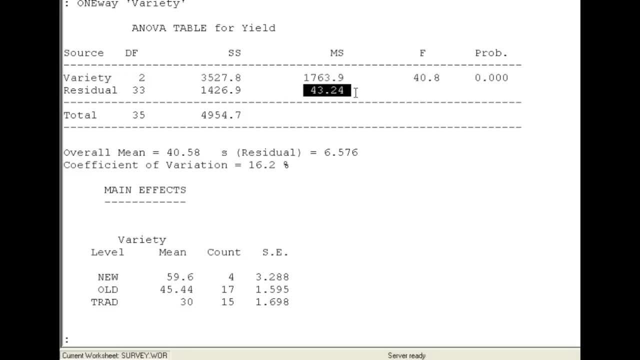 Below the ANOVA table, we have the S residual, in this case 6.576,, which is the unexplained standard deviation, ie the deviation in the data that's not explained by the variety factor. This is calculated as the square root. 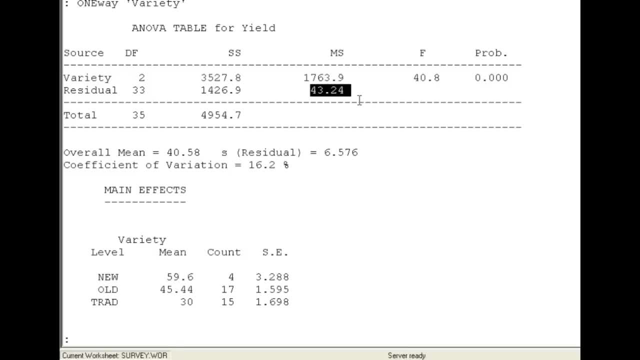 of the mean square for the residual. The coefficient of variation is the ratio of the unexplained standard deviation, 6.57, divided by the overall mean, 40.58, and that comes to 16.2%. The final element in these results: 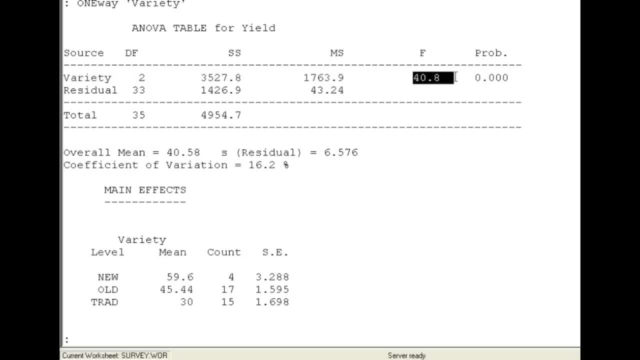 is the F statistic. This is a ratio of the variation between the groups, ie between the new, old and traditional, divided by the variation within the group. A large F value indicates more difference between the groups than within the groups. For this variety analysis, 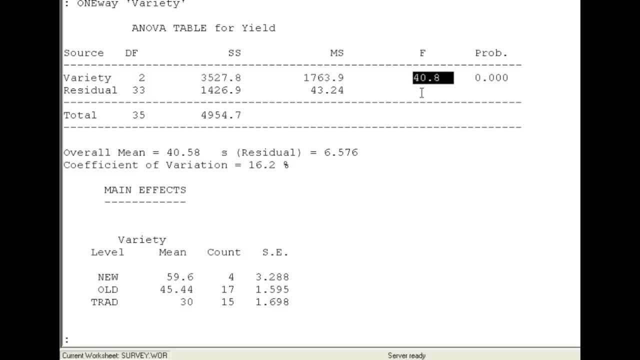 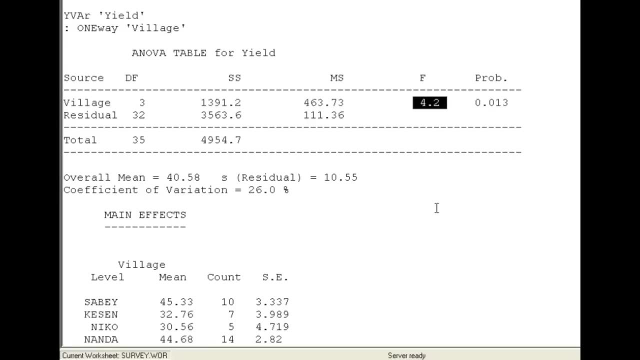 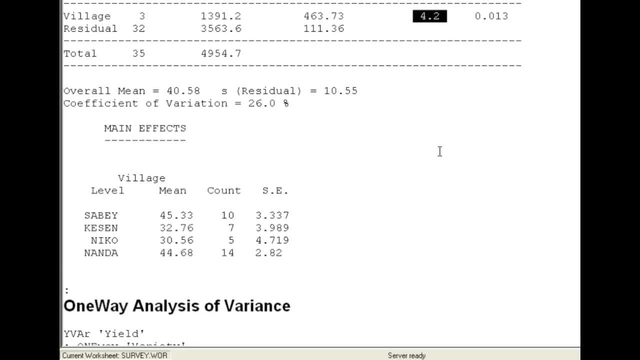 the F value is 40.8.. We look back to the village analysis. We find the F statistic there. the F value there was only 4.2.. This is further proof that the variety has a greater effect on the yield than does the village.